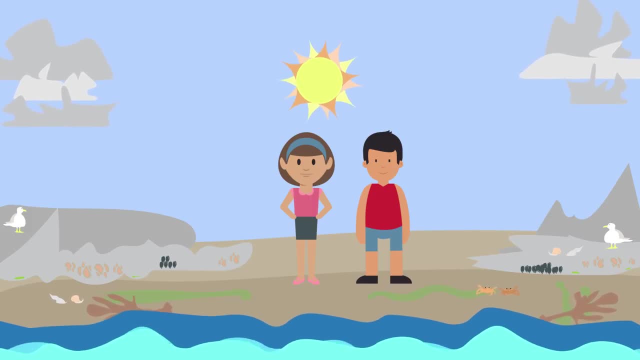 but we should count every single species along the shoreline. How long do you think that would take? Of course it would take too long. Instead, we sample a small section of the area, which gives us a representation of the whole area. Sampling allows ecologists to 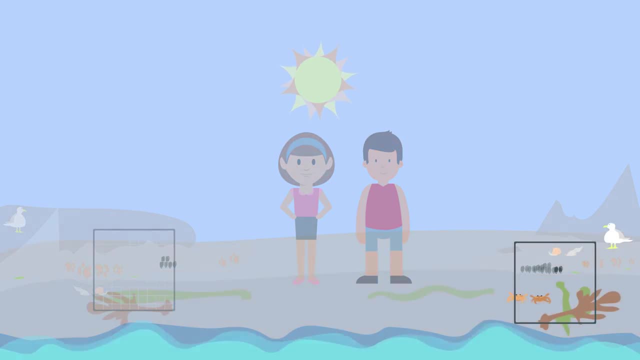 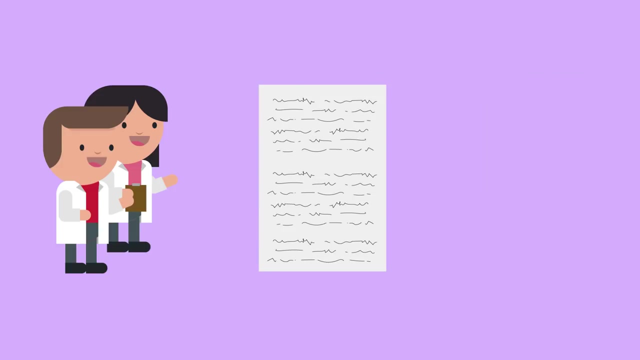 cover all the different areas within the habitat without having to record the entire habitat. This enables ecologists to measure the biodiversity of an area, record data on abiotic factors and even get a good estimate of the complexity of a local ecosystem in comparison to other. 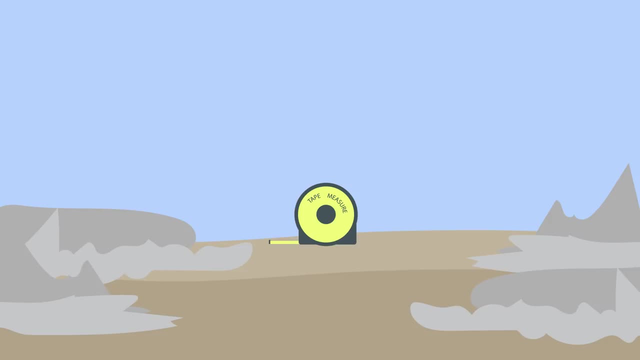 sampling sites On the rocky shore. we use a tape measure and one of these, a quadrant. Quadrants are square frames of a known size such as 1m2.. They could be like this or like this: We monitor sedentary organisms, So organisms like plants, algae, fungi and some animals. 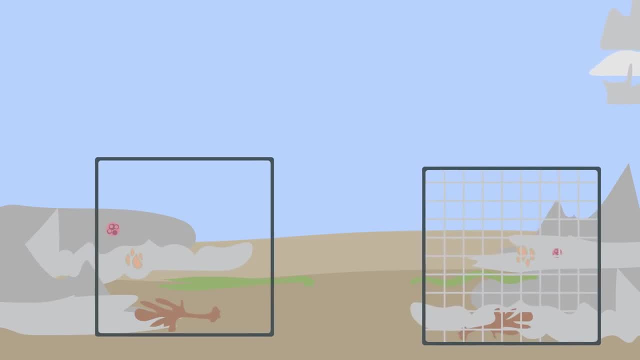 such as barnacles, which do not move about from one place to another. Perfect for us to study the shoreline At low tide. we place a tape measure perpendicular from the sea up the shoreline like this. This is called a belt transect. We have subdivided the shoreline into zones, kind of like a grid. 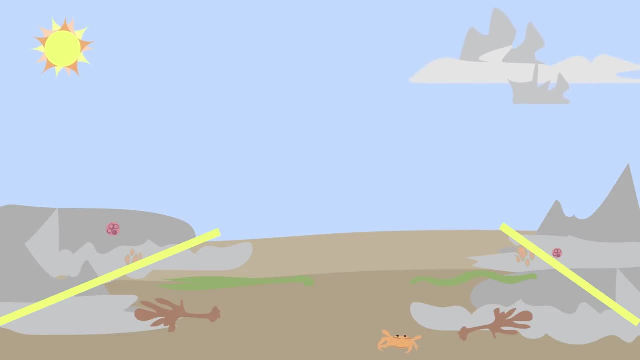 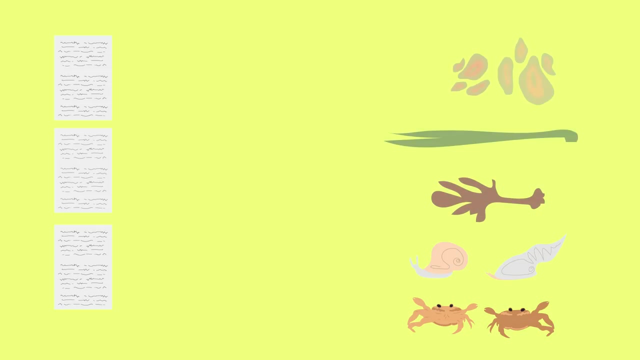 system to ensure that we sample the entire area fairly and don't get biased data. At regular intervals along a belt transect, we place the quadrants down and count the percentage cover of each different species found. This gives us information about how the population of different species change as we move up the rocky shore. From our data. 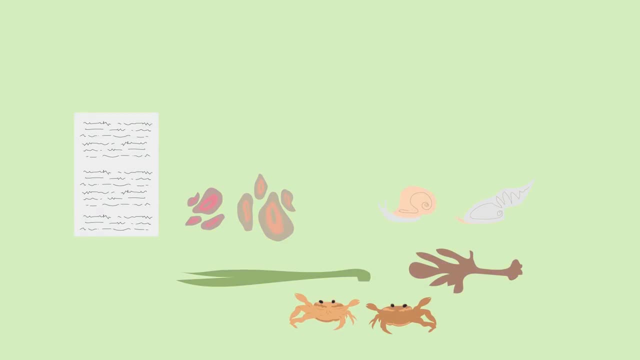 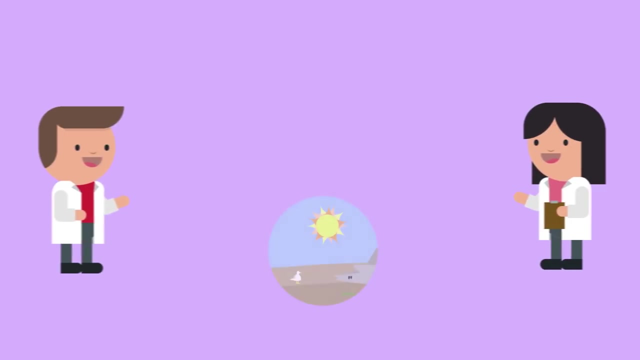 we can clearly see that different species can survive in different areas or zones along a shore according to the different abiotic factors. But ecologists don't just study rocky shores. They use a variety of different environmental sampling techniques. They use a variety of environmental sampling techniques to investigate. 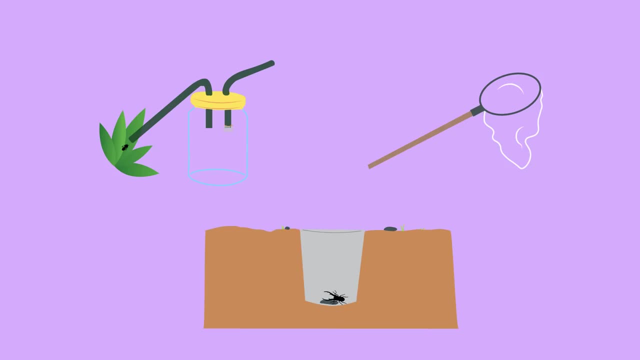 lots of different ecosystems. Here are some more examples of sampling techniques. This is a pooter which is used to catch small insects. Here is a sweep nest. These are used in areas of long grass to catch organisms. They can also be used in ponds- Pitfall traps. 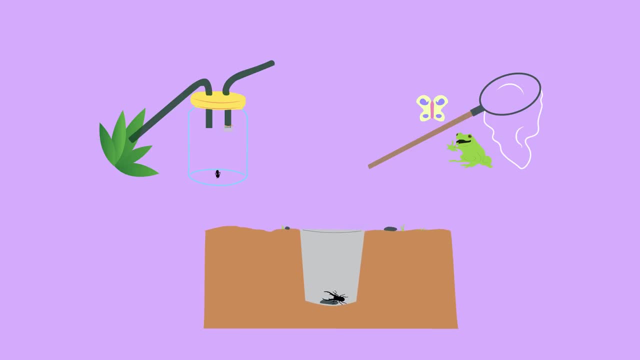 are used to catch small crawling insects and animals. They can be set up and left overnight to catch nocturnal species, For example to investigate how many beetles are in the area of a woodland, Or you might use quadrants to investigate how many daisies there are in a field. But